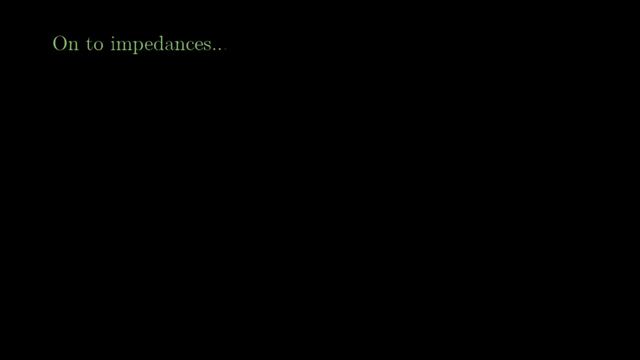 So there are voltages and currents, and we're two-thirds of the way there. The vector impedance is made up of two components. One is resistance R, which is the result of resistors, obviously. The other is reactance X, which is the result. 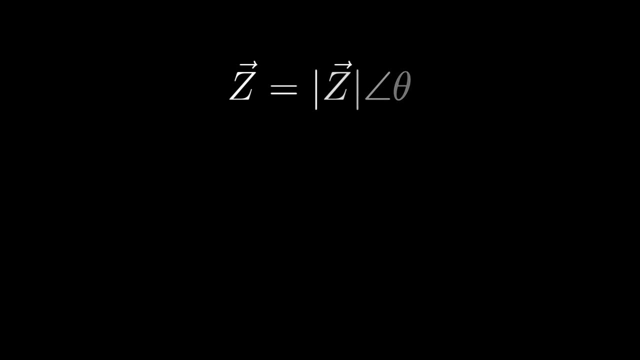 of capacitors and inductors. Now, unlike voltages and current phasors, we typically don't write impedance as a magnitude and an angle. Instead, it's broken up into its components. The horizontal I-hat axis is the resistance and the vertical J-hat axis is the reactance. 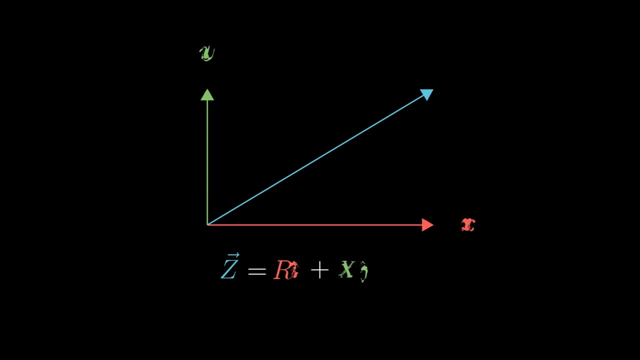 But instead of writing these in the XY plane, we're going to imagine them in the complex plane. The X axis is the real component, the Y axis is the imaginary component, And because electrical engineers already decided to use I to represent current, which stands for intensity, 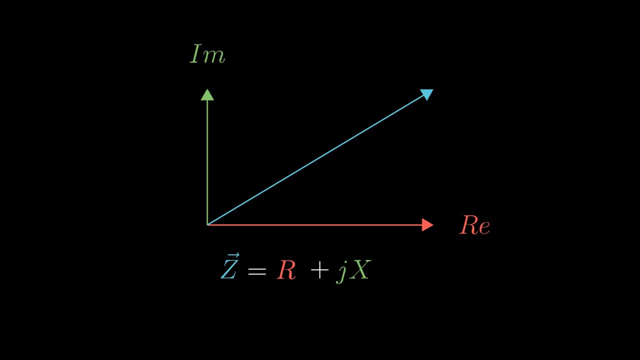 we will use J to represent the imaginary number, much to the scorn of mathematicians everywhere. So our 2D vector is actually a complex number. Let's look a little bit more into reactance In DC capacitors and inductors. eventually, 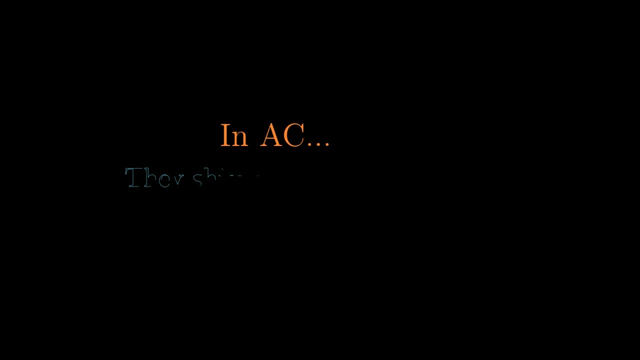 just become open and short circuits. But in AC what they do is they shift the phase of our waves. Capacitors slow the change in voltage so they make the voltage wave fall behind the current. They drag the voltage back, so the voltage is said to be like a wave. So 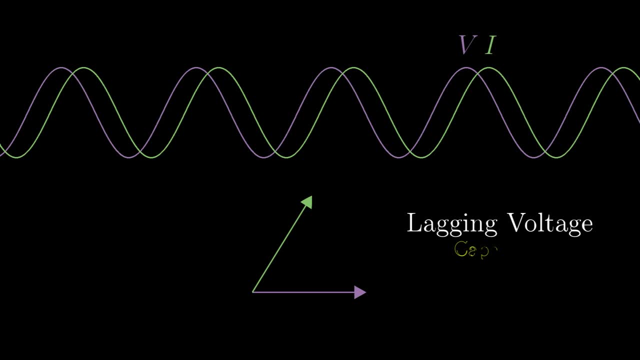 we're going to be able to see the change in voltage. So we're going to be able to see the change in voltage, So we're going to be able to see lagging. When you see this, you know the line is capacitive, With our phasors leading. 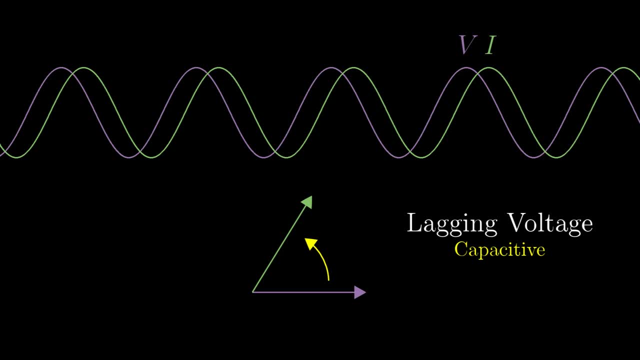 and lagging is measured in the counterclockwise direction, the more clockwise of the two being the leader. Conversely, inductors slow the change in current, so they make the current fall behind the voltage. In this case, the voltage is said to be leading and the line 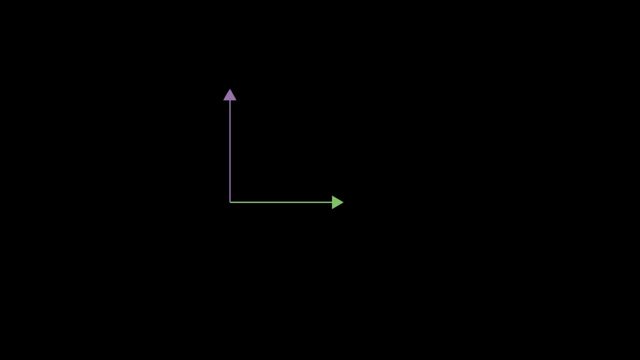 is inductive. You might be thinking: well, either could be leading or lagging, depending on your perspective. The voltage could be leading by 90 degrees or it actually could be lagging by 270 degrees, But by convention we just take the smallest angle.